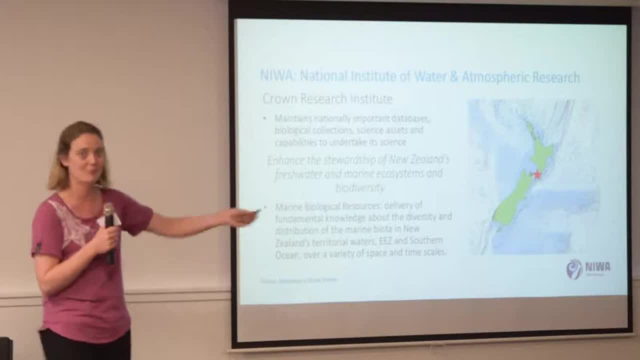 was for the conference participants to let them know where we were, because we were in Dunedin And the program specifically I work in is the Marine Biological Resources Program. So we're delivering fundamental knowledge about the diversity of life in the New Zealand territorial waters, but also down in Antarctica and a little bit of the Pacific as well over. 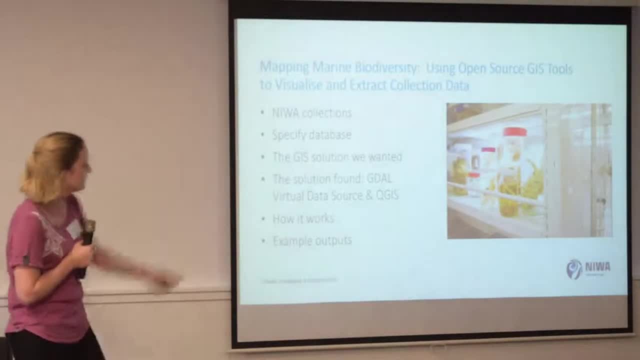 time and space. So a little picture of my collection there. I probably would have put more collection pictures in if I had more time. Basically, I'm going to give you a little overview of the collection, what it is a little bit about, what database we use, the solution we wanted. 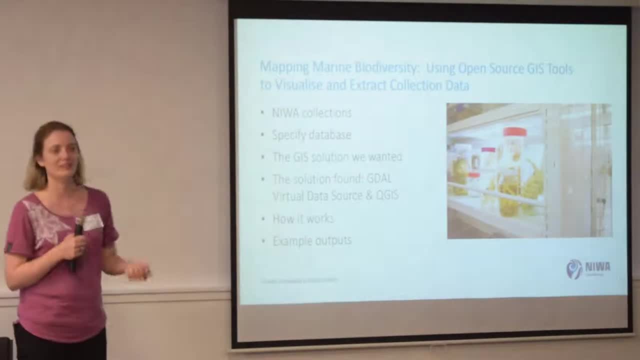 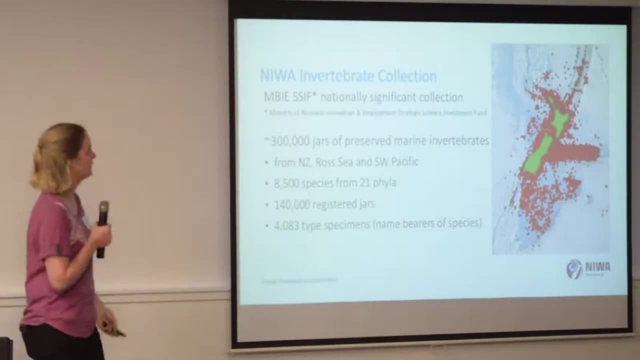 the solution that Brent helped me to find, how it works, and some outputs. So the NIWA invertebrate collection- lots of acronyms there. You don't need to worry about those too much. but MBIE funds us And we get funded under the Strategic Science Investment Fund And that gives us some money. 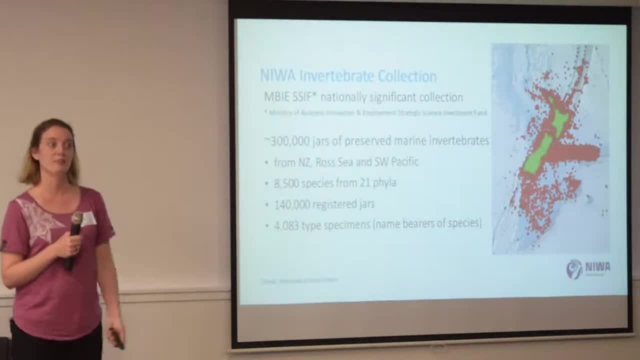 to look after the 300,000 jars of preserved marine invertebrates we have in our collection. So that's anything without a backbone. The fish go over to PAPA collection and we take everything else that's not a fish. Is this better? Thank you. 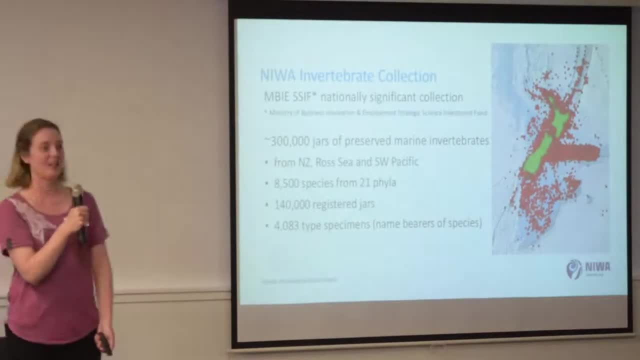 Okay. So, as I said, we've got animals from around New Zealand, the Ross Sea and the Southwest Pacific. We have 8,500 species in the collection and we actually only have 140,000 registered jars. So we have quite a lot of work to go to get everything into our database. So we're continually 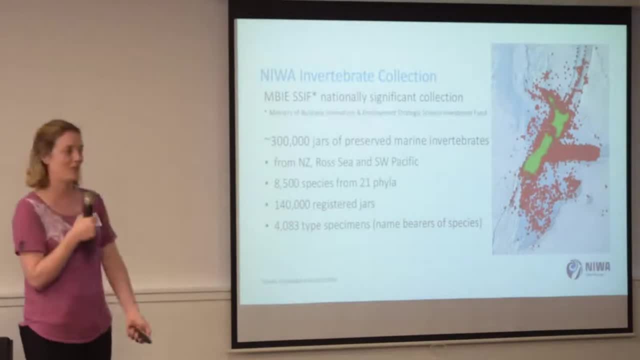 adding to it every day, but it's a long way to go until we get everything registered, This little output on the map on the edge there is all of the points from inside the New Zealand Exclusive Economic Zone. So lots of points around, lots of areas that are important. 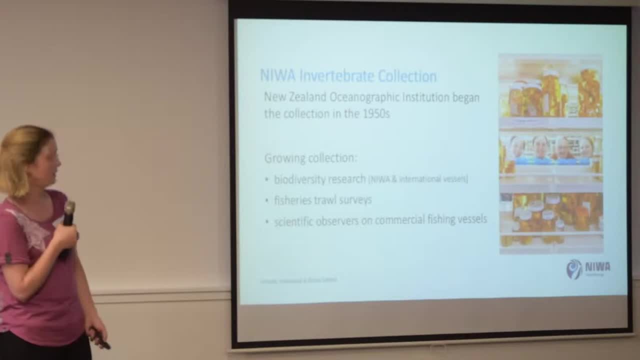 for fisheries. So the collection started in the 1950s and it started out with the New Zealand Oceanographic Institute collection And it's been growing ever since. We get samples from biodiversity research cruises. So that's where I go out and I we're answering a particular question. 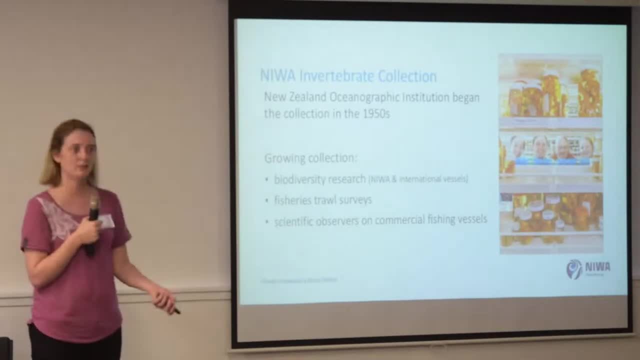 about a particular habitat, So maybe we're going to sea mounts or undersea volcanoes to learn more about the animals that live there. We also get samples from fisheries research: trawl surveys, So they're assessing fish stocks, So we get samples from the fish. research trawl surveys. So they're assessing fish stocks. So we get samples from fisheries research trawl surveys. So they're assessing fish stocks. So we get samples from fisheries research trawl surveys. So they're assessing fish stocks. So we get samples from fisheries research trawl surveys. So we get the bycatch. So everything. 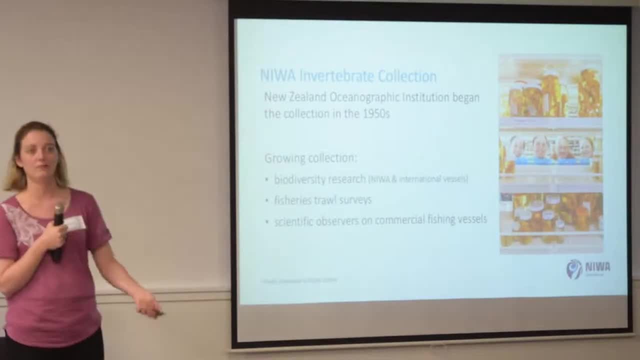 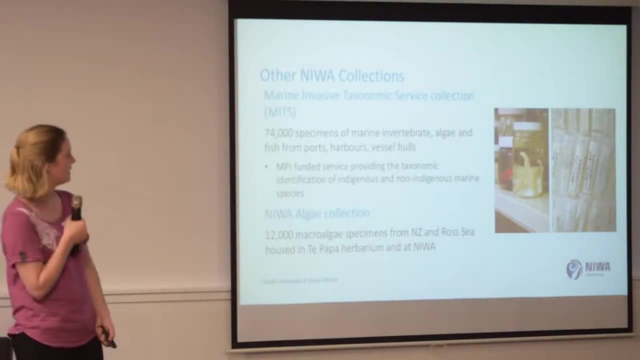 that's not a fish, And scientific observers on commercial fishing vessels send us samples as well. So that's a lot of data coming in to us from lots of places, And we also have the Marine Invasive Taxonomic Service collection, which has a lot of invasive creatures from 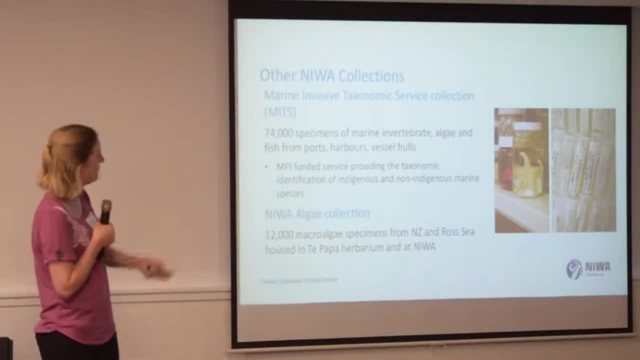 ports and harbours that we're looking for, and also native creatures from around those areas, And we have an algae collection as well. It's quite small and most of it's held at Te Papa, But we have some of the data at NIWA, So we look after all of that in a specified 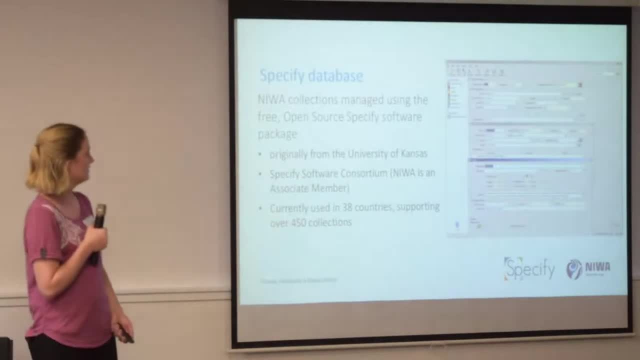 database, which is open source, And it's a really awesome piece of software for natural history collections management. It's got all sorts of great tables and fields in it that are very specific to what we do, So it's got locality information and preparation information. 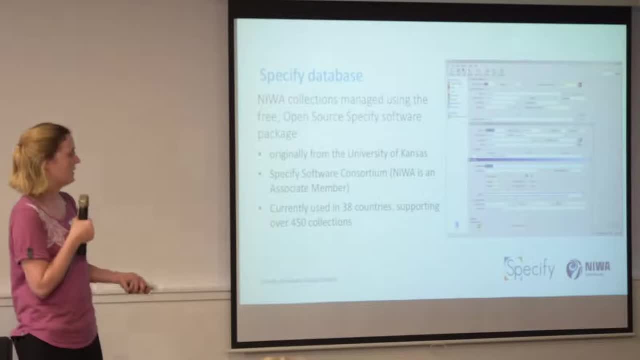 about how a jar is stored and where it's stored, And it has a big taxonomic tree behind it with all of the species names And the different levels of taxonomy. So it's developed at the University of Kansas And they now run it through a software consortium in which we've joined as an associate member. 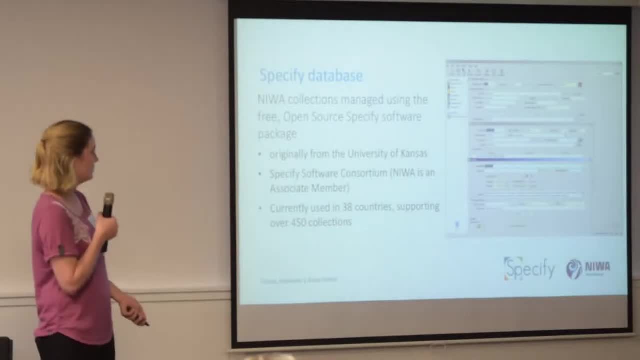 So we get a little bit of help if we have some problems, And it's used around the world in over 450 collections, So it's quite widely used and lots of people really like it. So it's a suite of applications with an underlying MySQL database And it 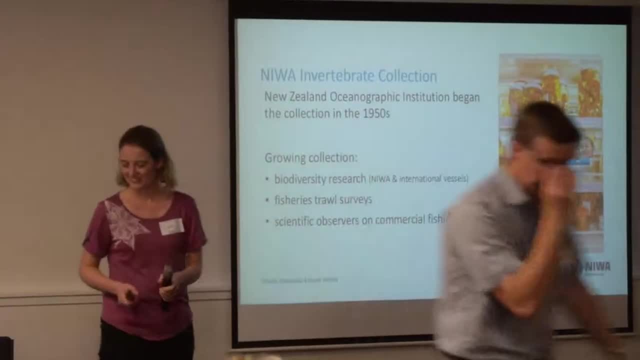 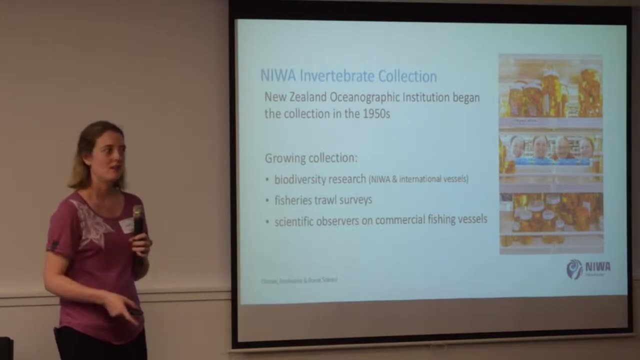 That's right, Yeah, Yeah. So they store their collections up at Torrey Street And they havethe National Fish Collection is there And they do have some invertebrates, But it's a much smaller collection of marine invertebrates than what we have. They have. 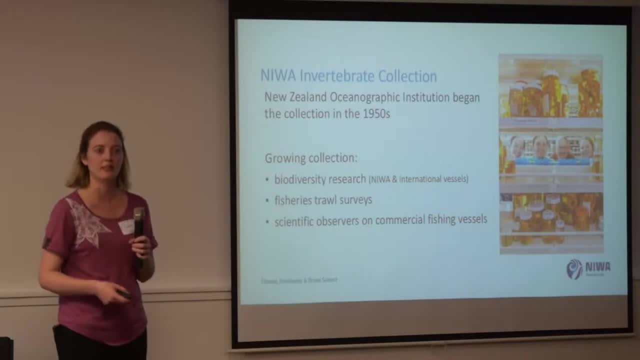 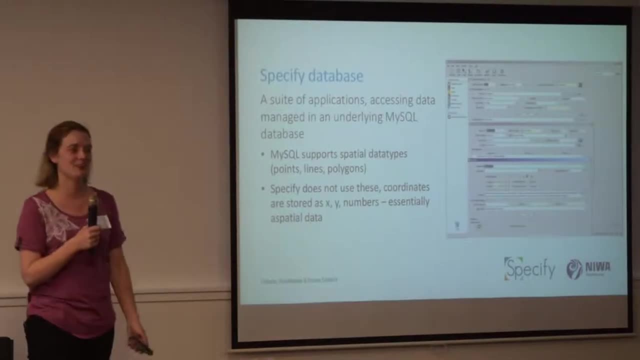 like a really massive insect collection and other invertebrates there as well. Yeah, Okay, So go back to MySQL databases. So they are spatial databases, So they are spatial databases, So they can store spatial points, lines and polygons within them And hopefully, 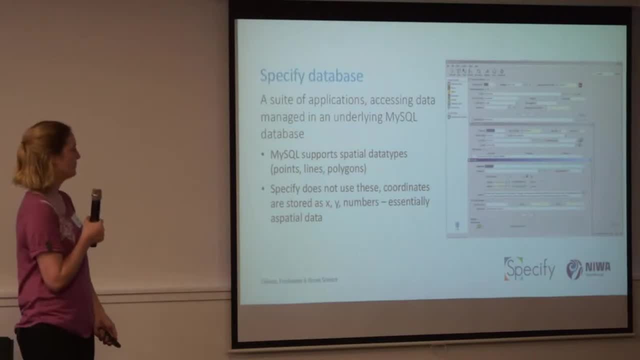 you all know what that means And specified, doesn't use spatial data, though it could. The coordinates are stored, So we have a latitude and a longitude coordinate And that's stored just like as an XY number in a field. in a table We can have points and points lat-long. 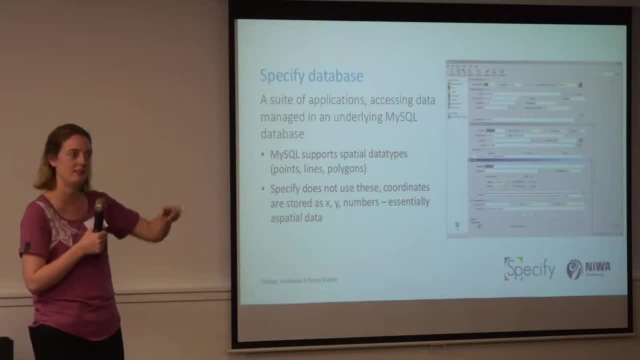 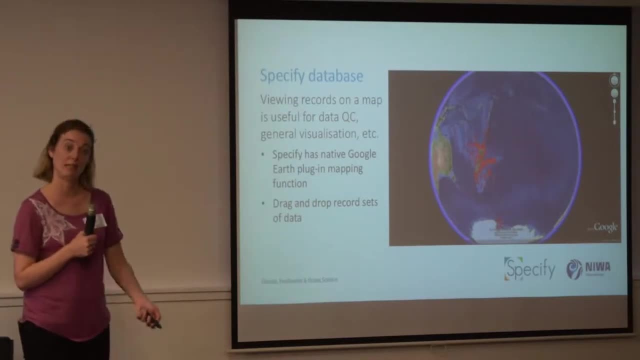 at the start and the end of a line. If we have a trawl we have a start and an end, So we can have points and points as well. So the specified database built in has a Google Maps kind of plug-in, So that's really great for visualizing data just really quickly. 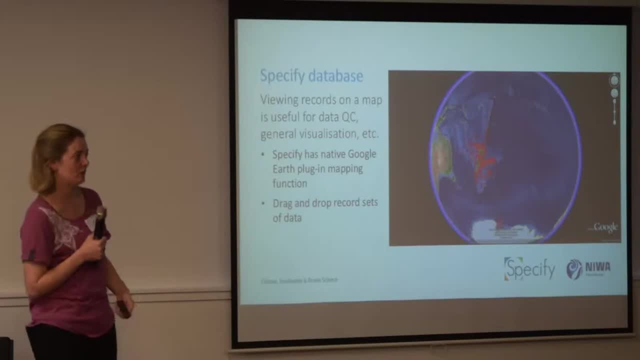 We can call up a query based on a particular species or a collection or a collecting event And we can drag and drop the data set onto the plug-in and it will open in Google Maps. That's really great for a quick look-in, Very easy. 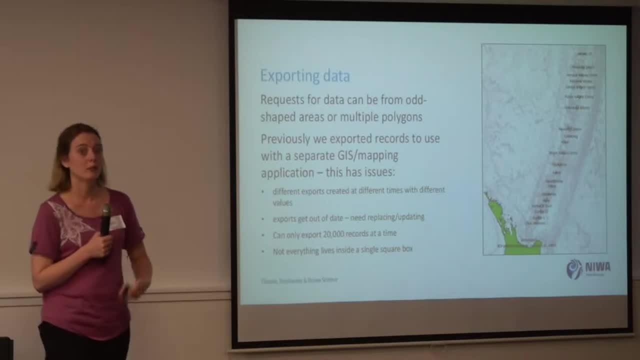 But we Often get asked for a little bit more complicated data exports And we also need to get asked to produce publication quality maps. So we need to use a GIS program towhich has got a little bit more functionality behind it so that we can manipulate a lot more of the 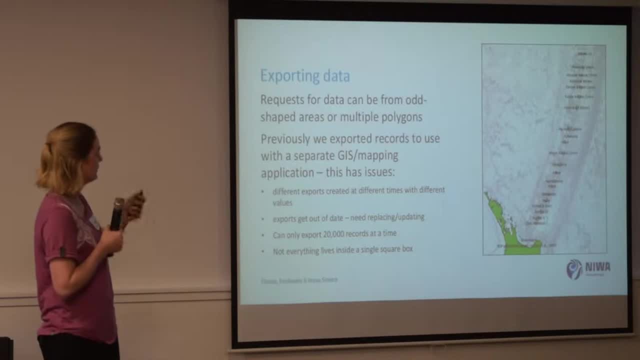 layers and add in layers and things. So we've been using QGIS. So we get a lot of requests for data from very odd-shaped areas. So this example that I've got up here on this slide screen is vent polygons. So this is areas on seamounts. They're undersea volcanoes which 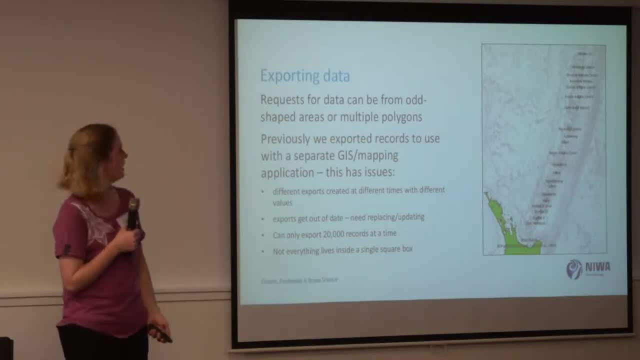 run up in a line up along the Kermadec Ridge And theyso we have ecologists that are interested what kind of animals living around these areas. So they made a request for all of the data that falls inside these polygons. So previously we would export that data. We draw a nice box around all of the records. 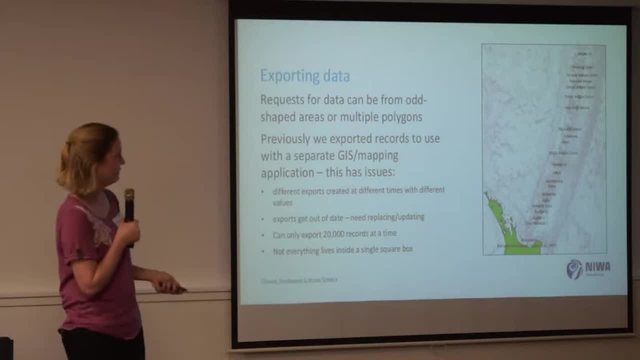 within the query With a query and we would just extract everything and then delete records out. that didn't quite fall in the area we thought- And there's a few issues with that- or we wouldor we would send it to a GIS person who would plug it into their program And we'd provide them. 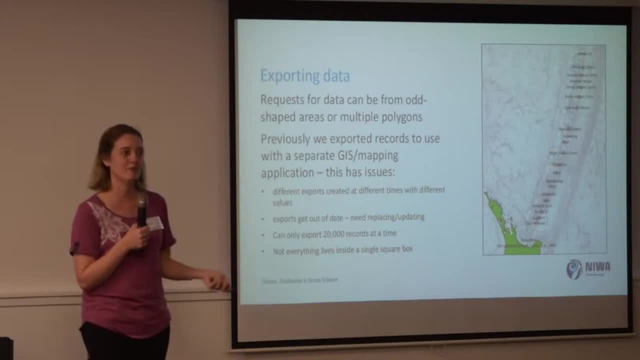 an export which was done on a certain date, so it's not live. If we made any updates, the export would get out of date. Or if someone identified a specimen, the name would change and that would mean the data was out of date. 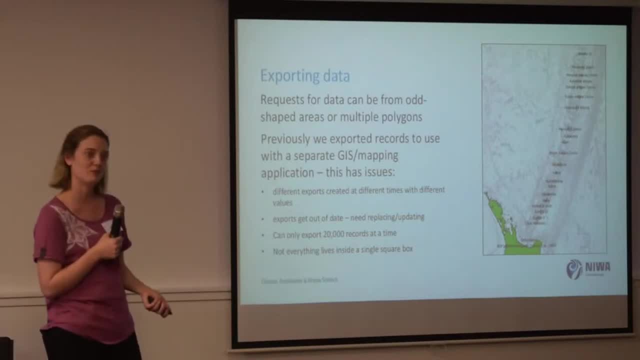 So we can also only export 20,000 records at a time and weI said we've got 140,000 records now. so that's very tedious. So it doesn't really work so well for us doing it that way anymore, and not everything lives inside a square box. 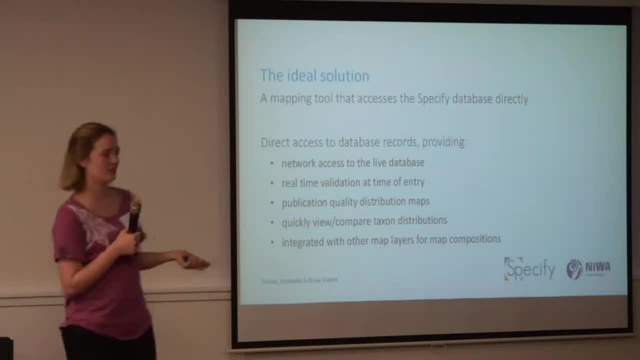 So the ideal tool that we thought we would like is something that gives us direct access to our database, So something that gets us right in there with real-time validation of the data that we're using. It can give us publication quality maps We can quickly compare and contrast. 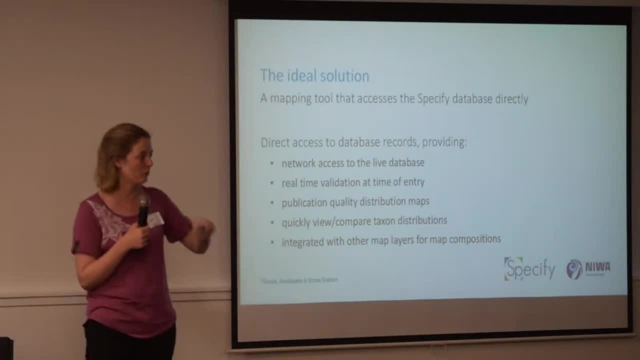 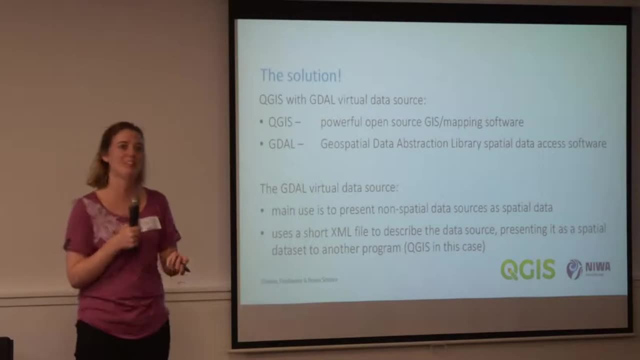 different taxon groups at one time. We don't have to export one at a time And we can integrate it with other map layers. So we came up with a solution- or I should say Brent came up with a great solution for us to try with QGIS and GDAL: geospatial data extraction library, spatial data access software. 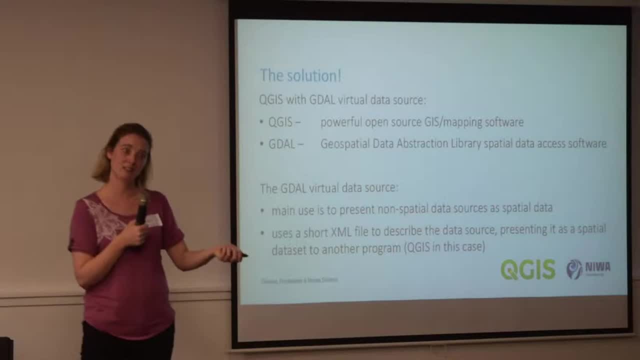 So it's a virtual data source which presents non-spatial data. So it's a virtual data source which presents non-spatial data access software. So it's a virtual data source which presents spatial data sources, like I was talking about our Latin long and spatial data, And it uses 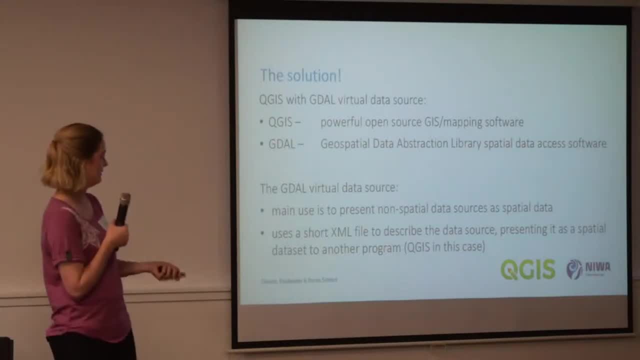 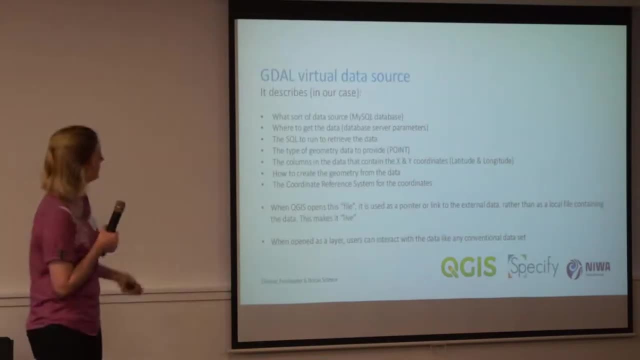 a file to describe that and where it goes to get that data. okay, So it describes. I'm going to show you the file that we used. So it describes what's the data source, where can we get the data, what our database parameters are the SQL. 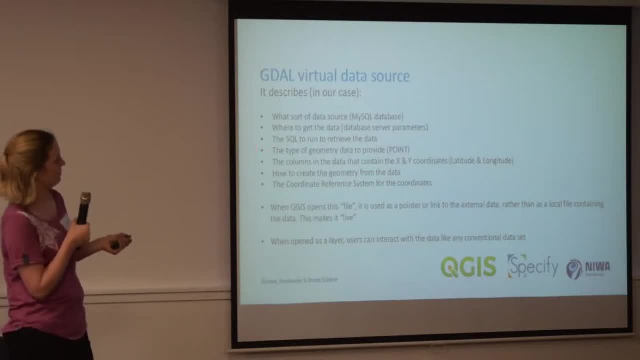 that it's gonna run to retrieve the data, the type of geometry data to provide the columns where they stay, database where the X and Y sit, how to create geometry and the coordinate reference system for the lat and long where it sits in the world. 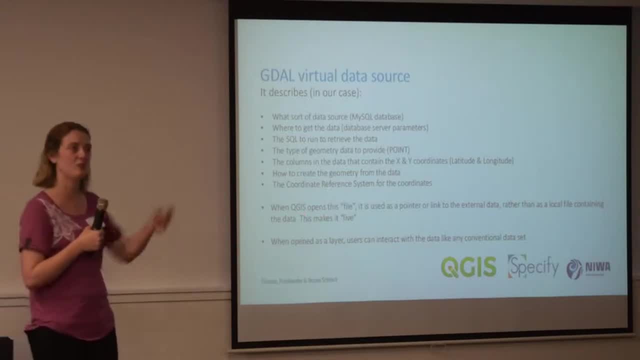 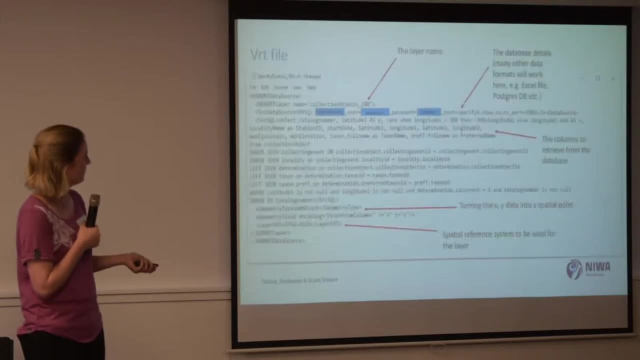 And this opens as a file. so it points to the data. so it's not the data in the file, so it makes it live. as soon as we enter something, it's updated on the layer already. So that's the file that it looks like, Just to show you. that's the name of the layer of our collection objects, our database details. 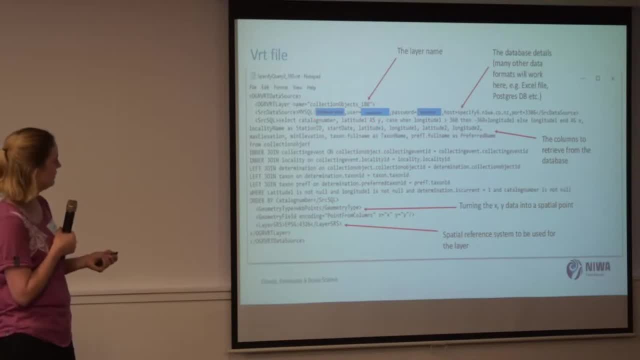 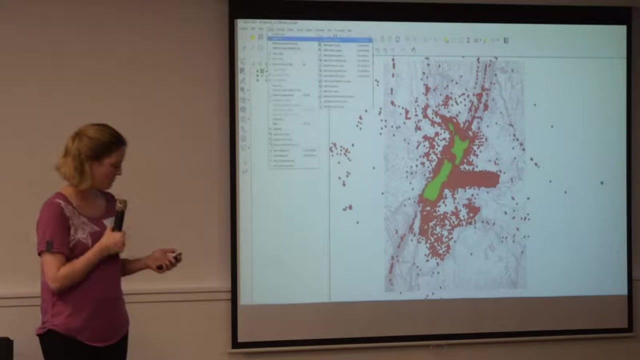 go in here and this is the query that selects out the columns that are relevant to the data we want to get out of the database. and this is how it gets it out of the database and just down here, the spatial reference coordinate system. So here's some screenshots from QGIS to show you what it looks like when we just load it. 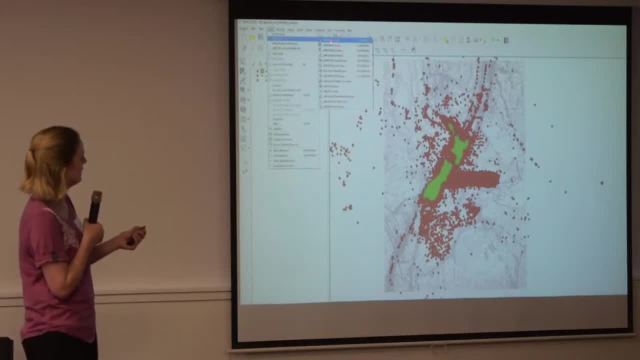 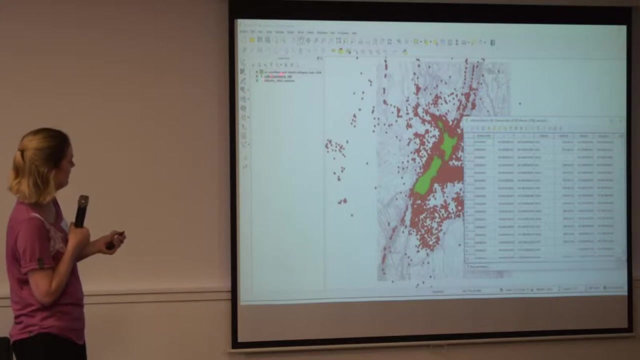 in so we can add the layer as a vector layer. so then we point to the where the file is on our computer And then it's just quickly live, grabs all of these points out of the database And if I right click on the layer, so up here is the layer in QGIS. 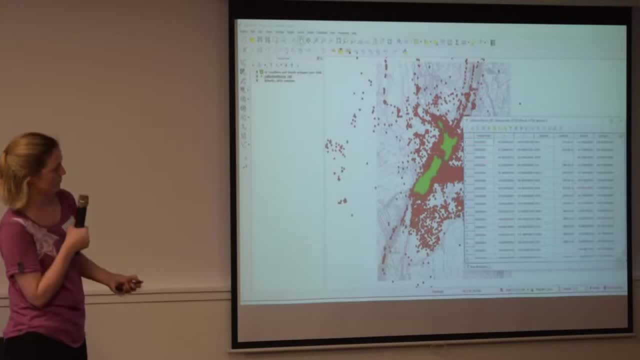 So if I right click on the layer it will open an attribute table and that's got all of my data in it. that's that I've asked for from the database, So I can add all of the fields in my database to that if I want to and get all of the data. 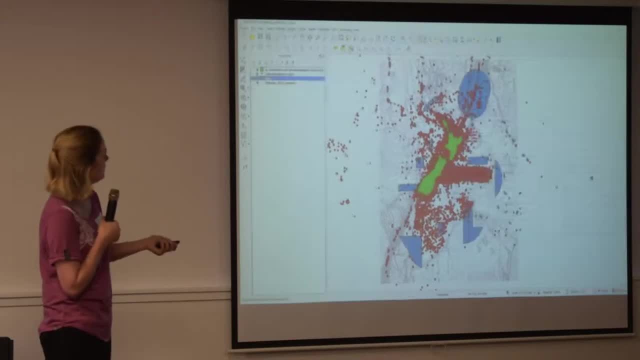 out into a mapping program which is really powerful. We can then layer on layers that Meaningful. so we have the layer here which is for bent thick protected areas around New Zealand. So for one project I had to provide a list of all animals that fall inside those areas. 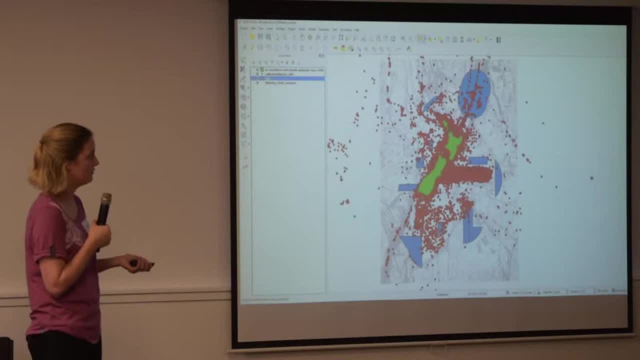 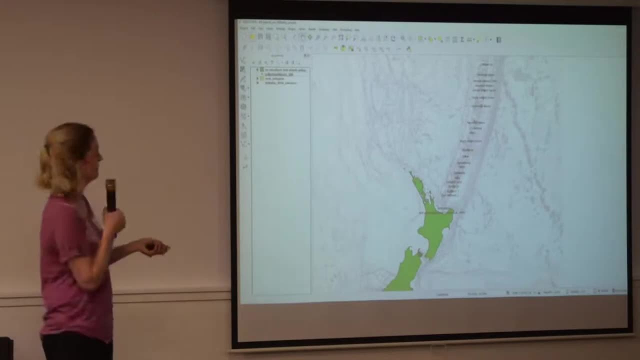 for the Department of Conservation and the Ministry for Primary Industries. And then again I'll just use my vent polygons as an example as well. Lots of different polygons on the map there, And I laid my data on the top And then we, And then we zoomed in to a couple of polygons there to show those records. 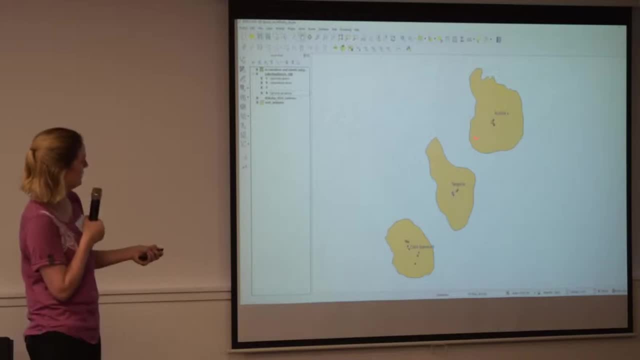 And just to show you, I can code with a little query the different species that fall in these areas. So I've turned on different species to show. So the top two here are ones that live around volcanoes and the bottom one here is a species. 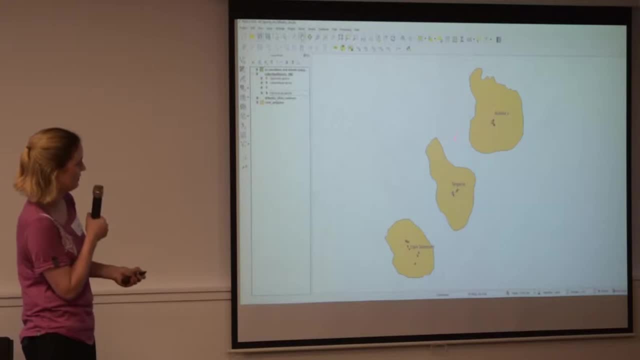 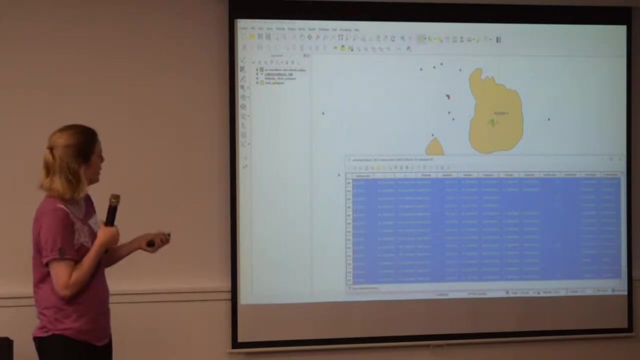 that doesn't Just to show like when we went to the seamount we found something with active venting, And when we went to this one we didn't. Okay. So you can start to do a little bit of analysis already, And also, when I want to highlight this, to get the data out of the map, I can use the 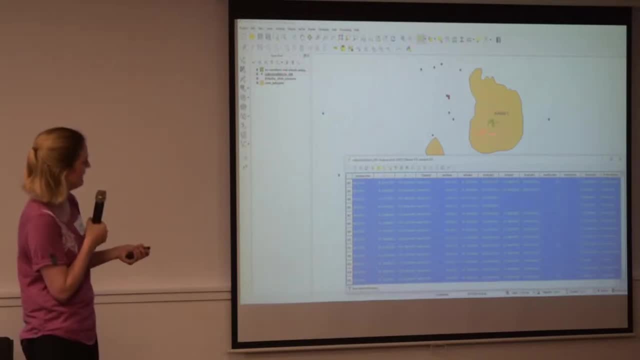 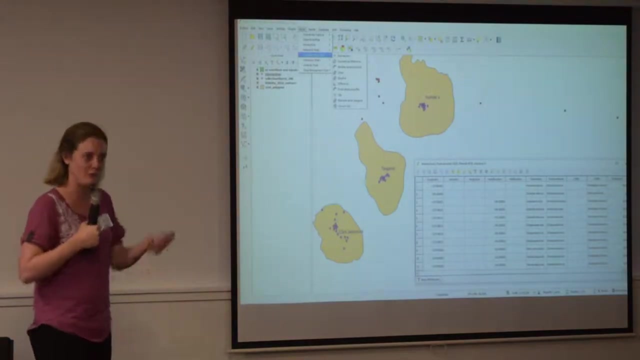 select tool and I can just draw around points in a polygon And when I right click on the layer it can show me the selected points and then I can export that and give it to the ecologist who wants the data really easily. And then if I want to get all of the data points from all of the polygons on the map, 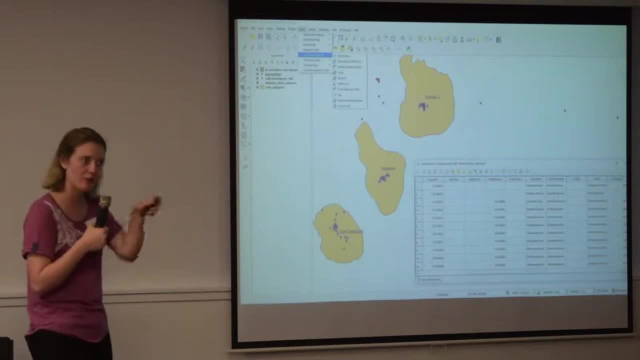 I can do that with a little tool. instead of dragging and drawing around boxes, around all the data, Using the vector geoprocessing tools, there's a tool called intersection and I can use that to give me a new layer called intersection, which is the intersect of with the data. 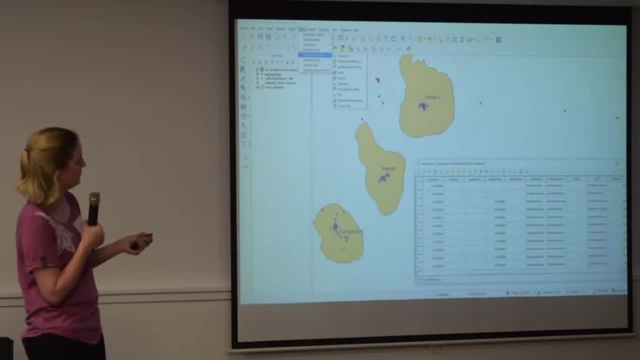 So it will make a new file which has got all of the polygon data and all of the data of the collection points that fall within it. So that's really now so powerful for me as a collection manager. So that's really now so powerful for me as a collection manager. 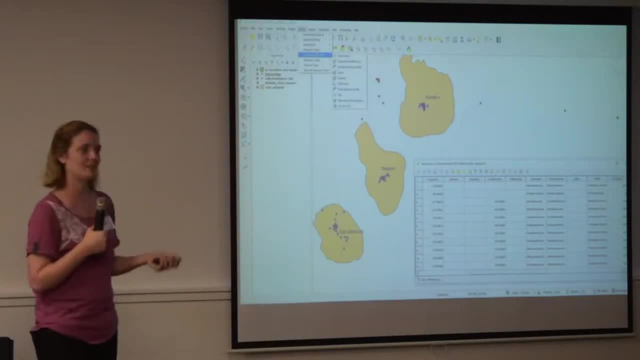 Okay, So that's really now so powerful for me as a collection manager. I don't have to go and draw around just one square area and then delete things out in my Excel file. It's a really powerful tool for me to analyze the data and pull it out quickly and then. 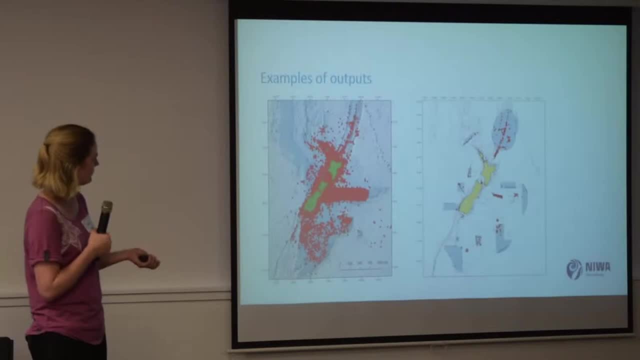 hand it to people that want to use this. So I mentioned before that QGIS can do publication quality maps. So now it means we can put all of our points on a map and produce something for a paper or a magazine article. and these are examples of some outputs. 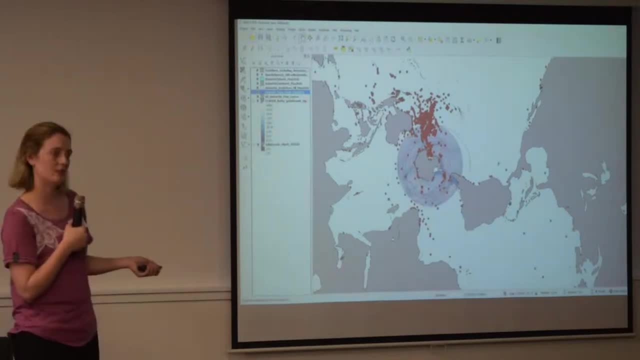 And also you can use different projections in QGIS so you can do a polar projection for your data if you've got data from around Antarctica, and here we always like to see New Zealand at the center or at the top. so we've got it organized so that New Zealand and the Ross 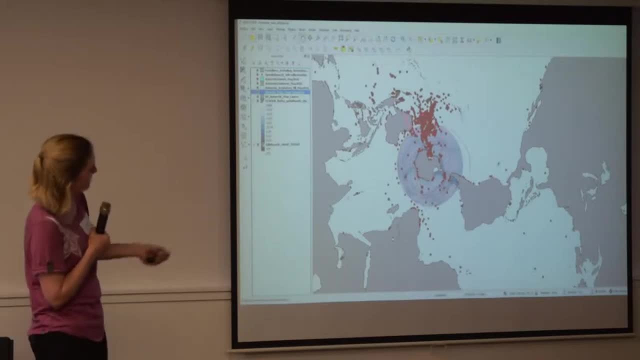 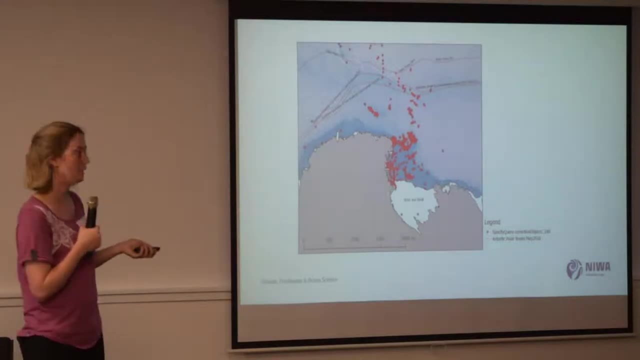 Sea, which is important to us, is lined up there and this is all of our points kind of on a world view of where all of our collections are from and a map that we produce just from the Ross Sea records. So it really was an ideal solution for us.